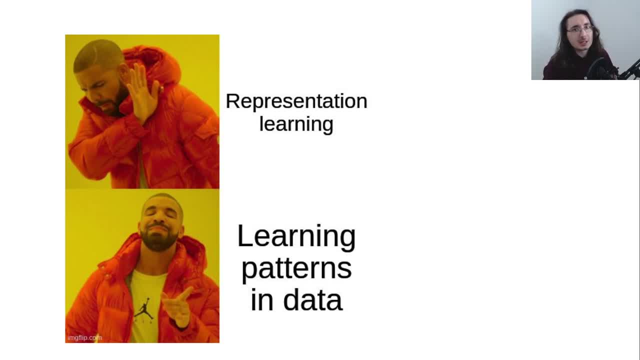 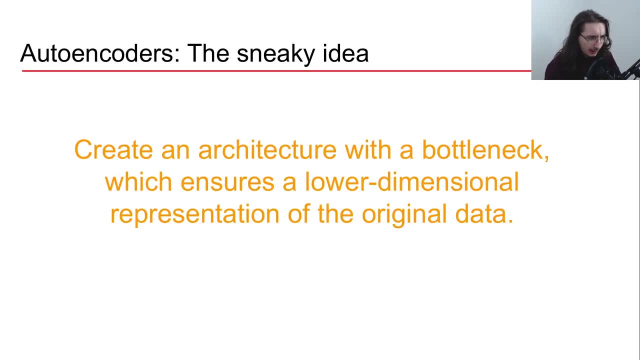 it's just learning patterns in data, learning structures that are present in a dataset. Okay, but now what's the idea that we have, like the basic intuition that we can use like which autoencoders to learn like this representation? Right, so I am straight to the translation. of learning patterns into the data. Hello to all the28 European states. Welcome, I'm Hasley. I'm Andrey Schalk and I introduce how to create a kun der Alt-e esimerk sweatshirt with the Microsoft Framework model, Visual Studio in para. All right, so at the end of this sing I want to partially fix and. 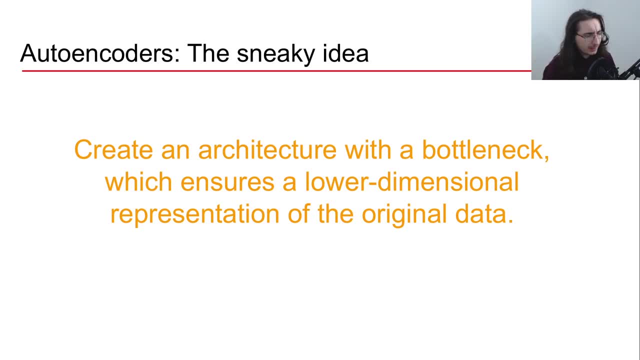 ending with a section on how to properly identify human conversation communications for even learning. Now I'll show you how to, too. representations of data. So we basically want to create an architecture that has a bottleneck and with the idea that this bottleneck is going to ensure a compressed representation of the 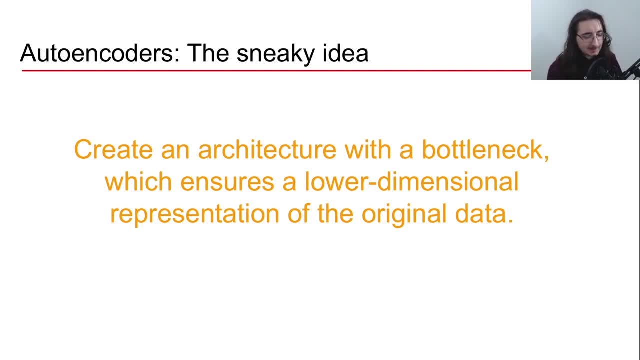 original data. Now, in this sentence, the most important concepts are bottleneck and lower dimensional representation, In other words, like this bottleneck is going to enable us to have like a compressed representation of the original data. I know this can feel a little bit like abstract, so now let's take a look at an example, at a visualization of an autoencoder. So here we have. 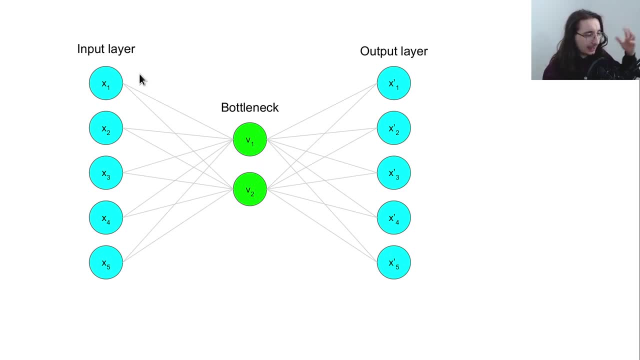 it and, as you can see, we have, like on the left hand side, an input layer where we just like feed in, like data, some kind of data. Then, at the center, we have this bottleneck and, as you can see, it's indeed a bottleneck because it 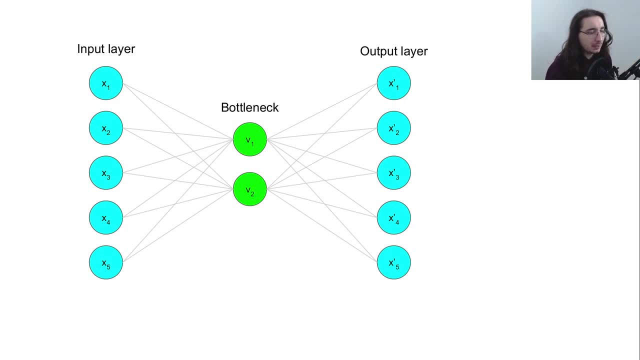 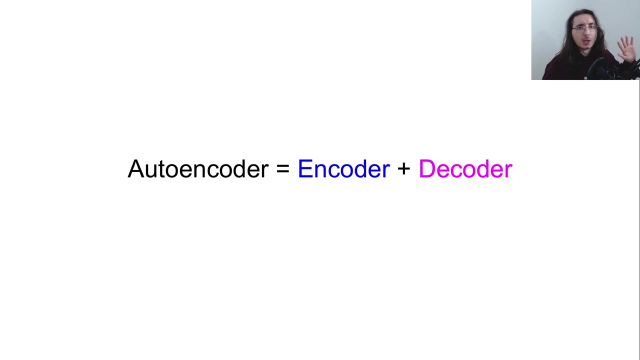 has a lower dimensionality when compared to the input layer, and then we have the output layer, which once again has the same dimension as the input layer. Now, an important thing to understand about autoencoders is that this is a quite complex network architecture that relies on two separate 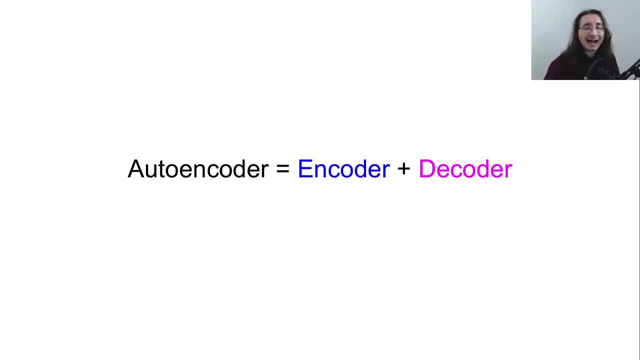 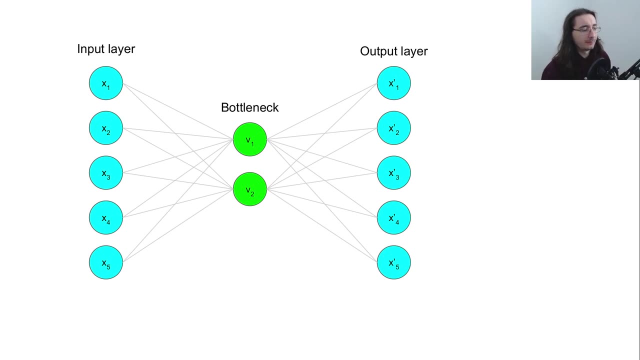 pieces. One is called an encoder and the other one is called a decoder. Let's try to visualize like these two parts. Let's start with encoder first. So this is like the encoder and its role is that of compressing data into a lower dimensional representation. In other words, we take like 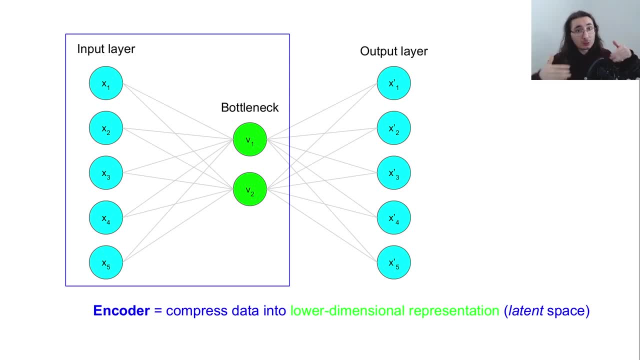 in the data as an input and then we learn weights so that we can compress down that data into a lower dimensional representation. This lower dimensional representation is often called a latent space, and a latent space is a representation of the original data which only focuses on the most. 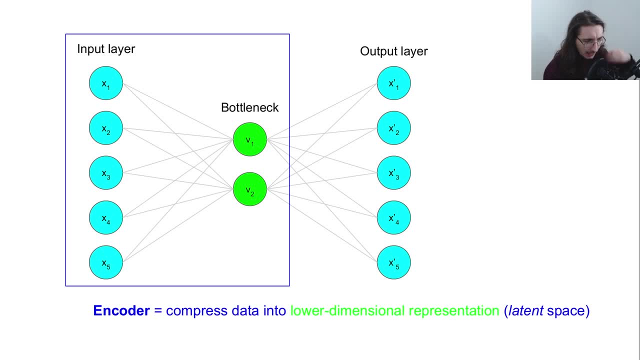 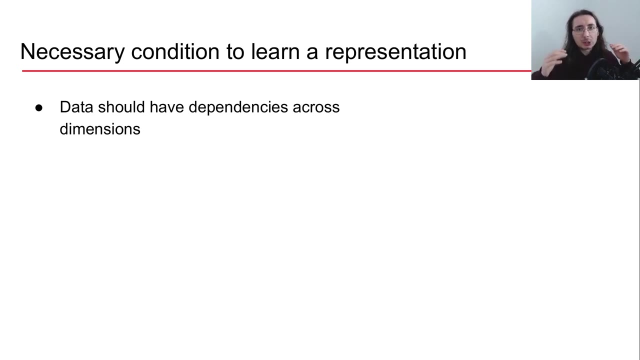 important attributes or features. Okay, but in order for the encoder to be effective at compressing data, we need for a certain condition to be true, and that condition is that data should have a dependencies across its different dimensions. In other words, if the different dimensions of the 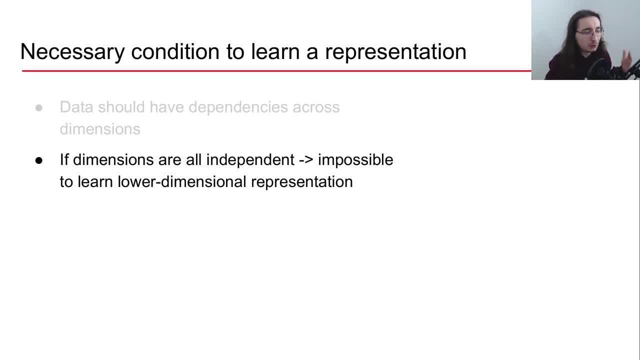 of data are all independent. it's basically impossible to learn a lower dimensional representation because there's no way of capturing most important, like attributes, without losing a lot of information. Okay, now you may be wondering: but is it an encoder, some kind of like dimensionality reduction algorithm, and is it comparable to other algorithms like, for example, PCA or principal? 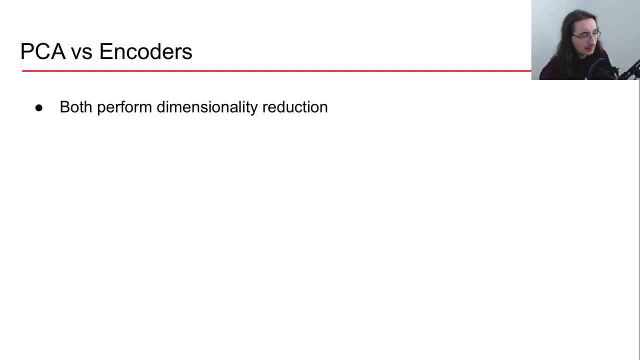 components analysis. Well, in a certain sense, yes. So they both PCA and encoders. they both perform dimensionality reduction, but PCA learns linear relationships, whereas encoders can learn non-linear relationships. Now let's take a look at an example in 2D so that we can understand how PCA and encoders like. 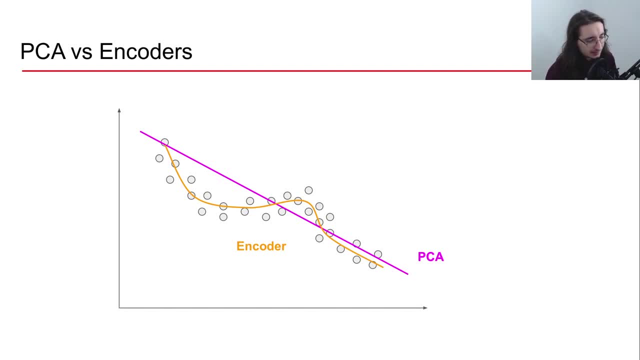 work differently. So here we have like our data and, as you can see, like our data is just like all of these dots. so with PCA we can fit the data only with a line, whereas with the encoder we can have a non-linear curve like this that follows like the, the data. 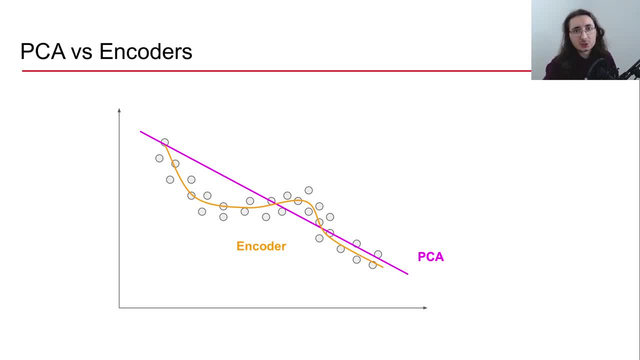 fits the data better. We can generalize this to as many dimensions as we want. In other words, PCA, even in three, four or five dimensions, can only capture linear relationships, whereas encoders can capture non-linear relationships. What does this mean? Well, it means that with PCA, we can only 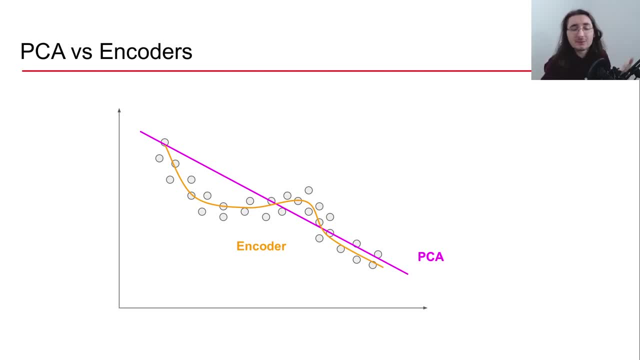 try to like compress data that has a relatively simple structure, whereas with encoders we can capture relationships in data that has like more complex structures. But the cool thing here is that if we were to use a linear activation functions in an encoder, then the encoder wouldn't. 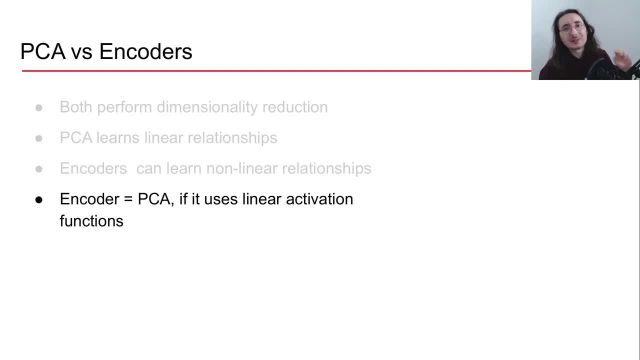 necessarily behave so differently from PCA because, at the end of the day, it would learn a linear representation of the data. So the advantage that an encoder has is that it uses linear activation functions. Now, if you're not familiar with activation functions and like these terms like are quite new to you, I highly suggest you to go check out my series called Deep Learning. 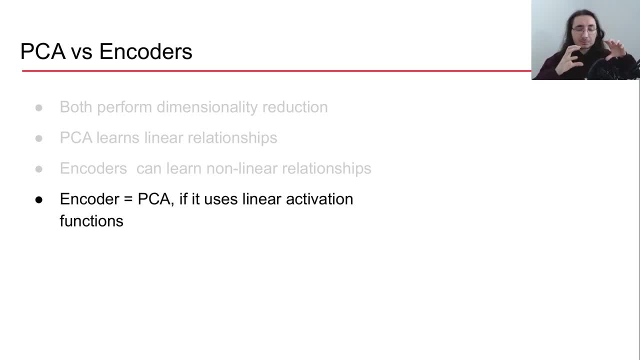 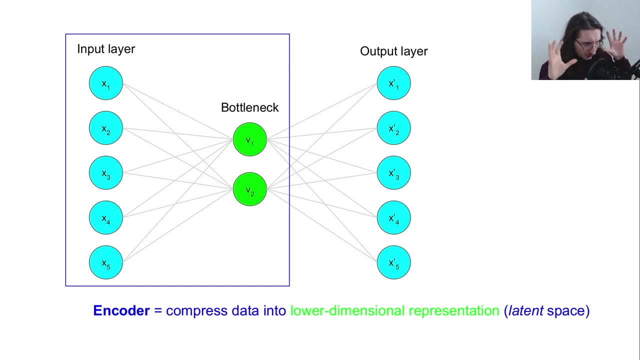 for Audio with Python, where I just tackle all of these concepts in deep learning from scratch and I also create like implementation in Python of this. Just check out the video or the series up here. Okay, now let's go back a little bit To encoders. so, as we said, like the, the role of the encoder in an autoencoder is that of compressing. 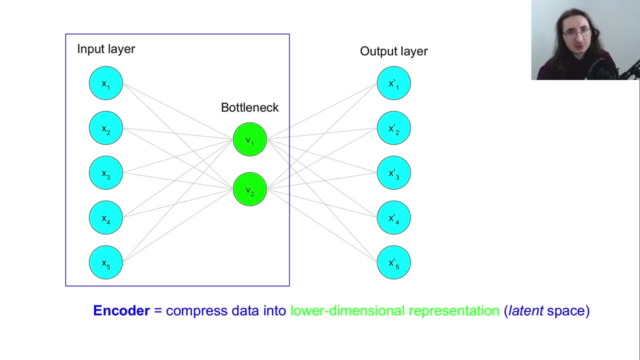 initial data into a lower dimensional representation and learning that representation. Now, what about decoders? Well, decoders, just like, do the opposite of that. In other words, a decoder decompresses a representation back to the original main, So it starts from the representation, from the lower dimensional representation. 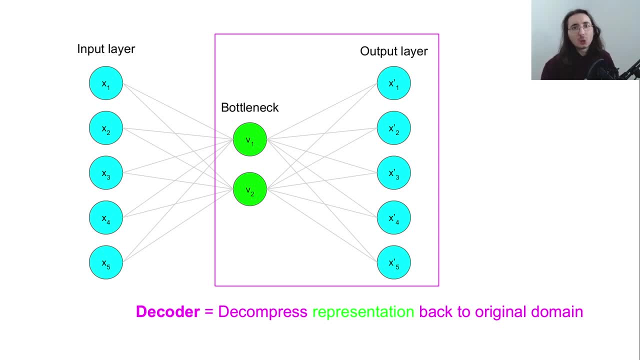 and then it tries to reconstruct the original data. Okay so, as you can see, like in an autoencoder, we have like this kind of like mirrored like image where, like the encoder compresses down data into the bottleneck and then the decoder like decompresses it up to, like the original dimension. Okay so we can like take a look like: 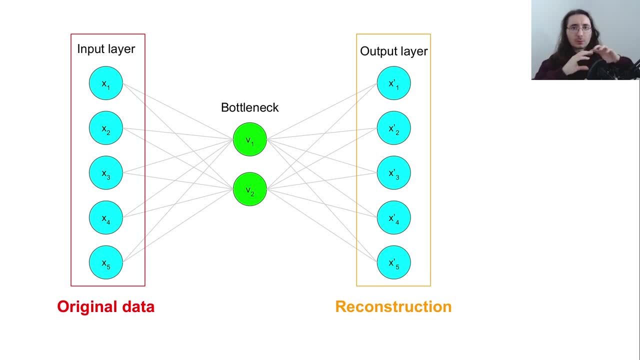 at this autoencoder and imagine like the whole workflow like this: So we start with the original data or like the input, then we just like represent it here down in the bottleneck or in the latent space, and then here we have a reconstruction of the original data. 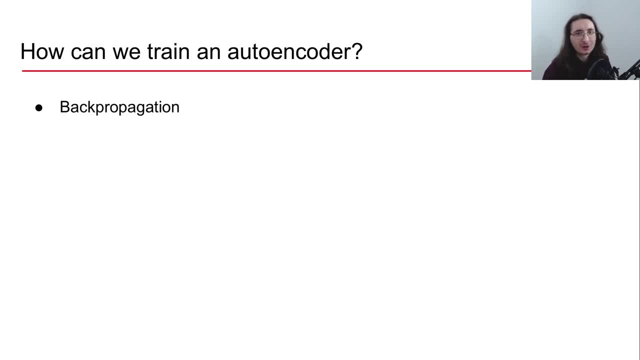 Now the question is: but how can we train an autoencoder? Well, for training an autoencoder, we use- as it's usually the case with neural networks, we use backpropagation. Now I'm not going to discuss the details of backpropagation, and if you're not familiar with that, I highly 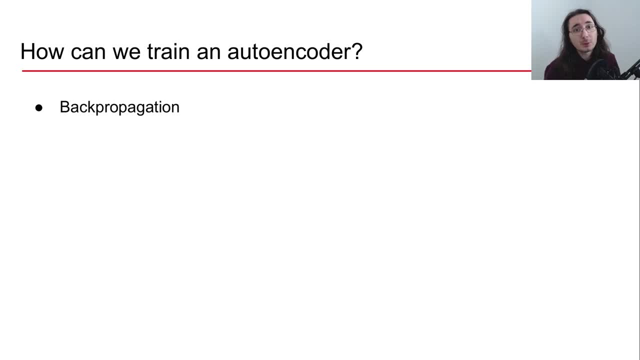 suggest you to go check out this video in the deep learning of Ferrodi with Python series. But the basic idea of backpropagation is that we need a way of like optimizing the learning process, and for that we need an observable. let's call it this way: 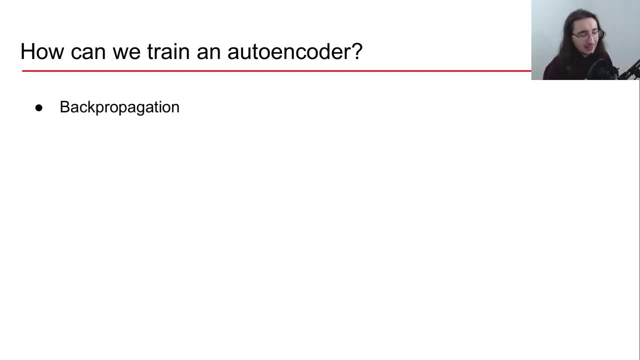 that's called loss or error. In the case of autoencoders, what we use is a reconstruction error, and the basic idea is that we want to minimize the reconstruction error. But what's a reconstruction error? Well, we can indicate a reconstruction error like this, and here we have the original data and here we have the reconstructed data. 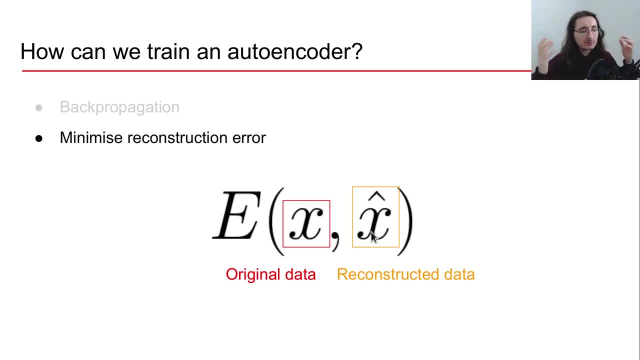 and the reconstruction error is, conceptually, the difference between the original data and the reconstructed data, in other words, is the difference between the input data and the data that gets spit out from the decoder. so we can take the difference there and so that we have an idea of how different the reconstruction is from the original data, now we can use a number. 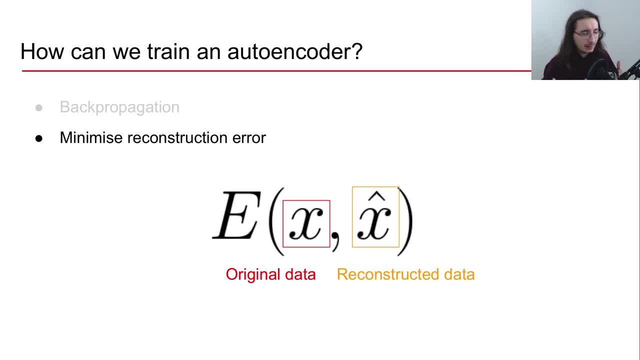 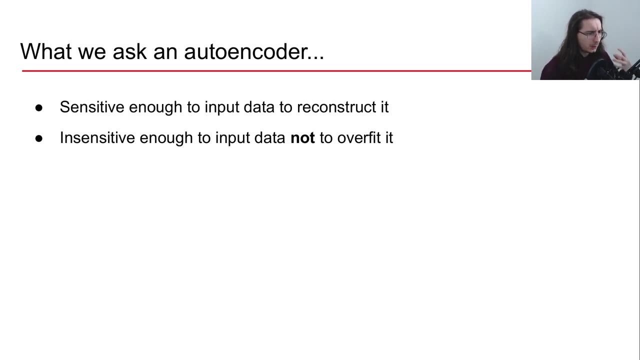 of different functions for actually like implementing the reconstruction error, but one that is usually used is a mean square error, msc or rmsc, which is a root mean square error. okay, so now what's an ideal or autoencoder? so what are, like the features or attributes that this autoencoder should have? 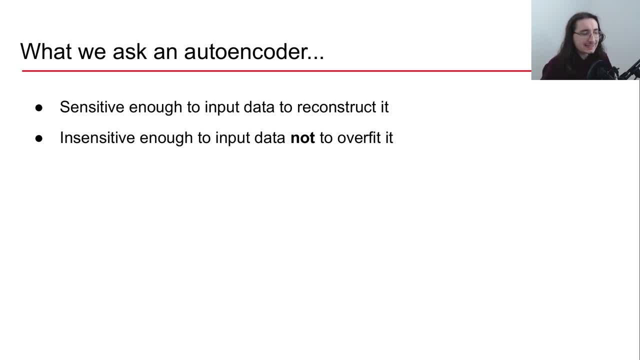 well, we want for an autoencoder to be sensitive enough to the input data so that it can reconstruct it, but, at the same time, we want for an autoencoder to be insensitive enough to input data so that it doesn't memorize it, so that it avoids overfitting it. right, and this is like a 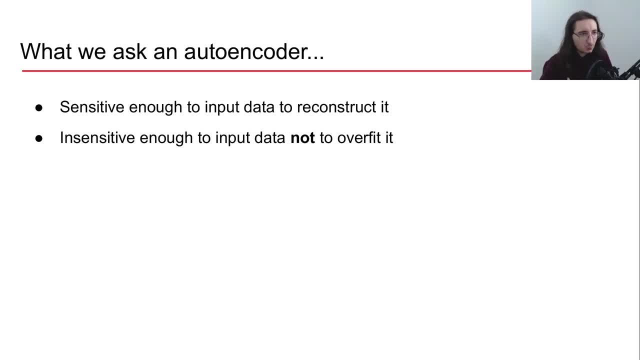 difficult trade-off to achieve because on the one hand, we want to- uh, we want for the autoencoder to learn a representation that represents well like the original data. so we have that representation that we can use to reconstruct the original data in a way like that satisfactory, but at the same. 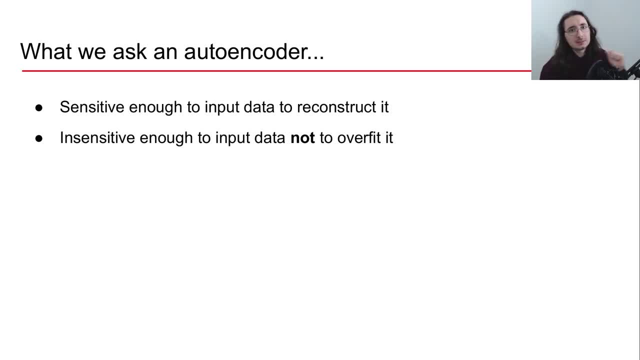 time. we don't want to learn all the unnecessary details of the input data. so this like looks like a mission impossible, but in. but actually it's quite fair to say that we don't want to learn all the necessary things to reconstruct that data and that as well. so the first one, we are going to do it. 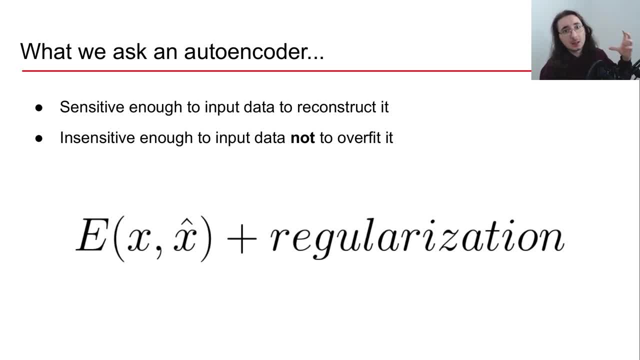 is I'm going to show you is actually a function that we're trying to construct. so, even if it's the most basic типа development problem we want to do is we want to be very sensitive to this type of representation and it's really just to make sure that we keep doing this. um well, 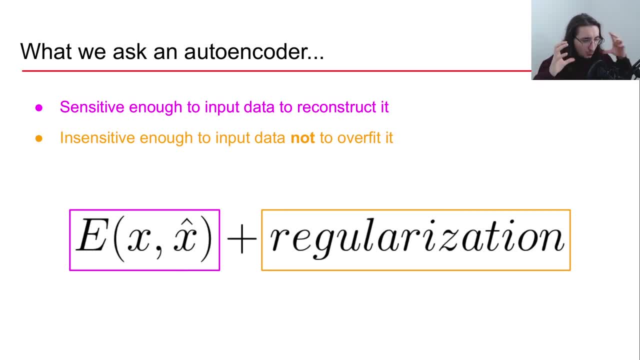 when we broke then to after with the reconstruction error. but things need to be a little more riff, improve with the reconstruction error. so the reason I should actually show you this is- and then I would show you a little moving around of things I'm going to show you and then it's possible- 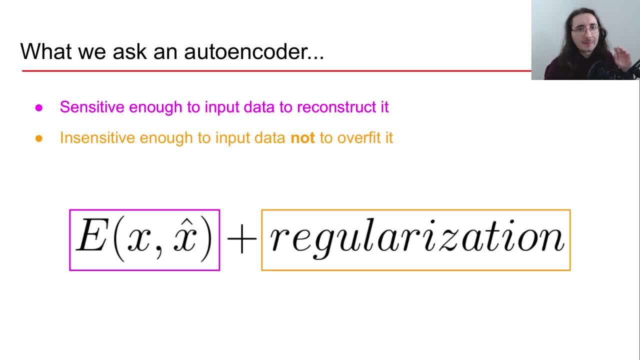 to the input data, so that we'll ensure that the network actually learns a representation that makes sense and can be used to reconstruct the input data. But at the same time, we need to add a regularization term, which will help us avoid overfitting the input data. Now 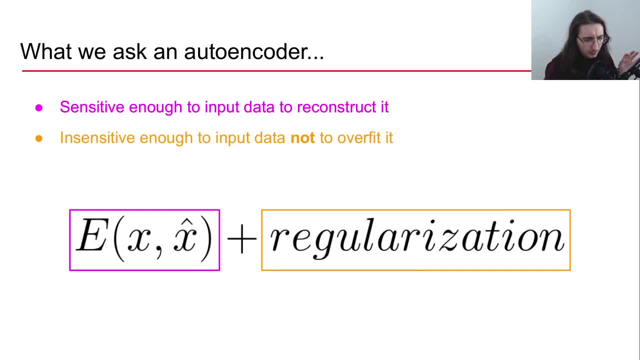 in the autoencoders. I'm not going to talk about regularization too much, but this is going to be a very important topic when we'll arrive at the upgraded version of an autoencoder which is a variational autoencoder. Just bear this in mind for future. 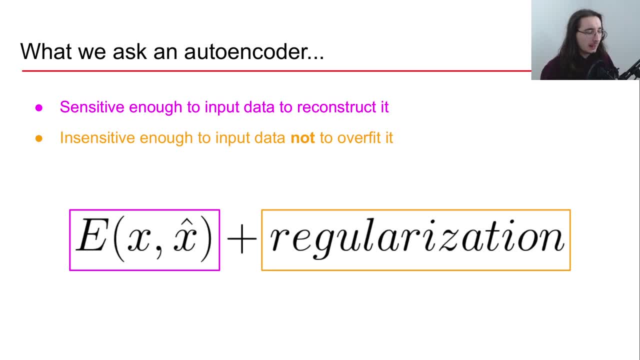 videos. There are two parts to the loss function. for the loss function, The first part is for the, an autoencoder, and one is the reconstruction error, and the other part is regularization elements which we need in order to avoid learning or overfitting the data. 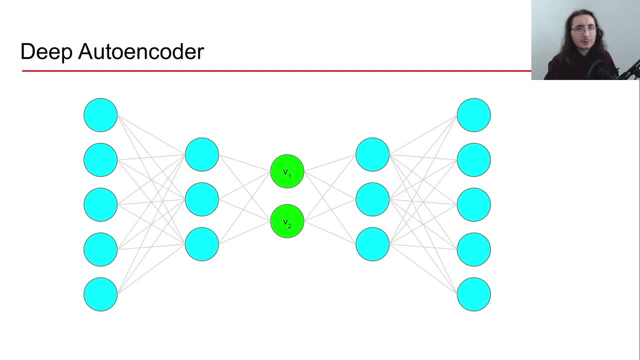 Okay now autoencoders can have deep structures. and what do I mean by deep structure? Well, as you can see here, they can have multiple layers before arriving at the bottleneck, and usually you have a structure that looks like this. So you start with: 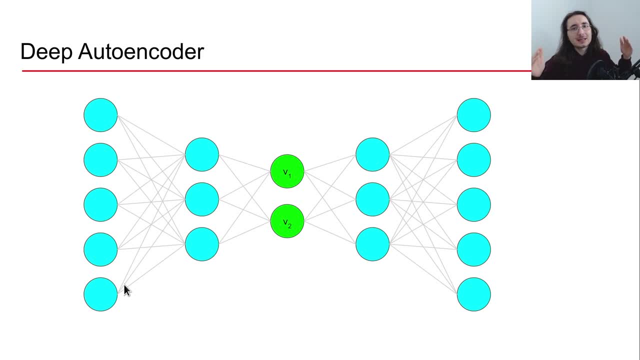 a lot of neurons, for example, and then you just go down to a layer that has less neurons, then less neurons, and in the end you arrive at the bottleneck. but as you can see here, this structure between the encoder and the decoder is completely mirrored. 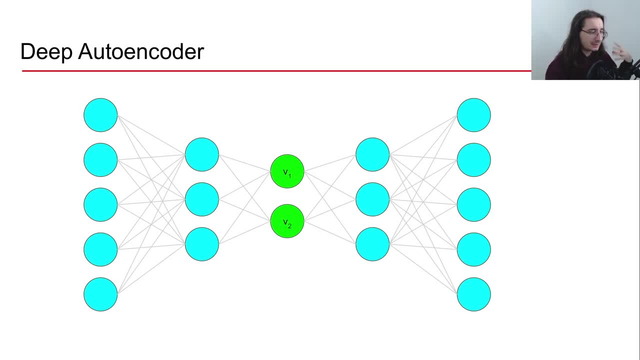 And this is usually what happens with autoencoders. So we start with the encoder, layer after layer, we reduce the dimensionality of the data until we get to the bottleneck, and then in the decoder we just do the inverse of that. So we start upsampling the data until we get to the output. 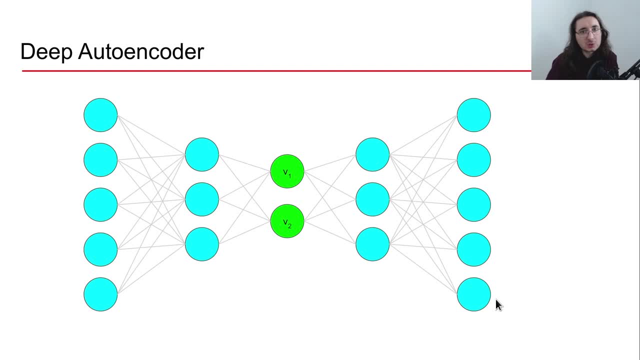 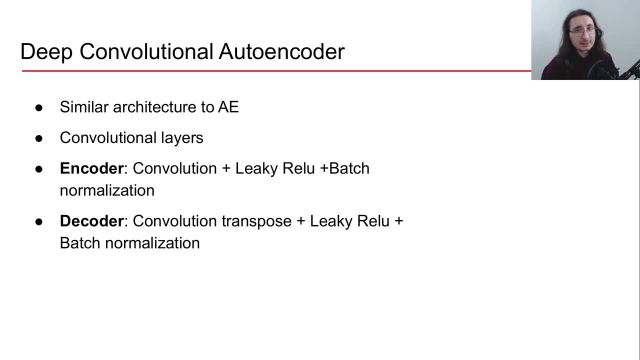 which, in most cases, has the same dimensions as the original data. Okay, so one flavor of autoencoder that's very important and is the one that we'll be discussing the most is the so-called deep convolutional autoencoder. So this obviously has like a similar. 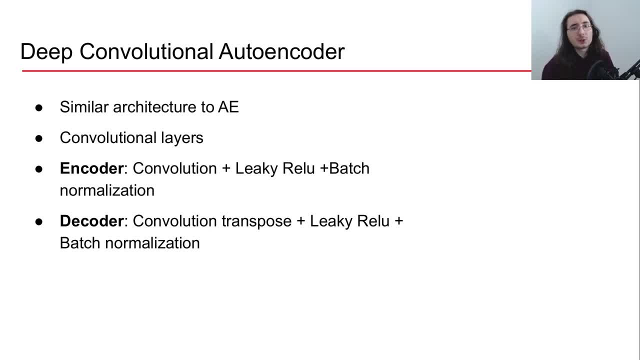 architecture to a normal autoencoder, a vanilla autoencoder. but instead of having like perceptions, it has like convolutional layers. And here, in the deep convolutional autoencoder still, we have the encoder part and the decoder part. At the level of the encoder, each layer. 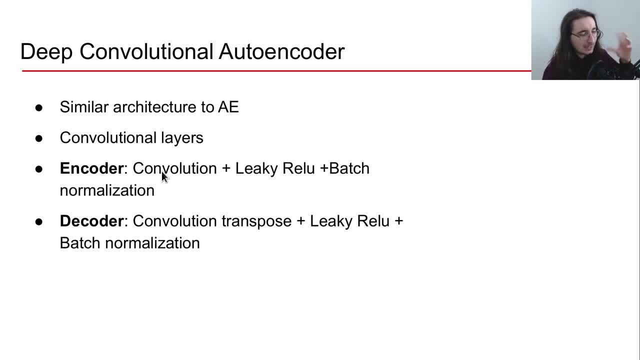 is a block that we can kind of like imagine having like three different parts. So we have like a convolution. we use a leaky relu or a leaky rectified linear unit as the activation function, and then we also apply batch normalization. So this happens at each layer in the deep convolutional autoencoder. 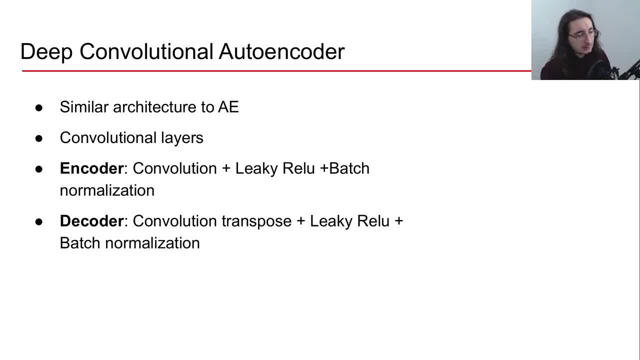 Then, when we get to the decoder part, what we have is yet again like a complex structure where we have like a convolution, but it's not convolution, it's the convolution transpose. Now, why do we use a convolution transpose? Now, why do we use a convolution transpose? 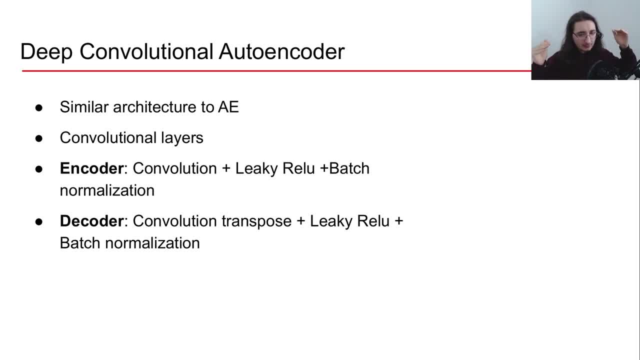 The idea is that using convolutions, we can kind of like downsample the data, compress it. With a convolution transpose, we just obtain the opposite effect: We upsample data, and that's what we want in a decoder. Okay, so in the decoder, at each layer we have a convolution transpose. 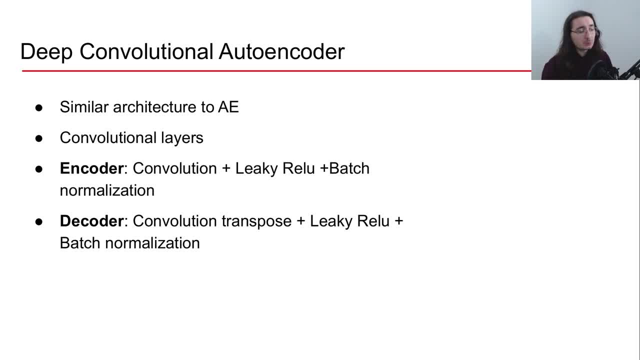 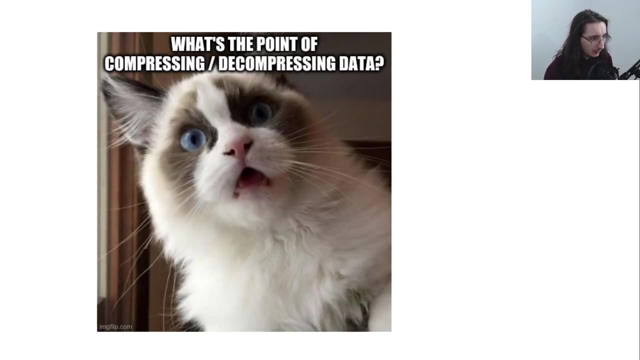 then again we have leaky relu and then we also apply batch normalization. So it's not always the case that you have like these elements in a deep convolutional autoencoder, but most of the time this is like what you usually get. Okay, I'm sure now you had like a very 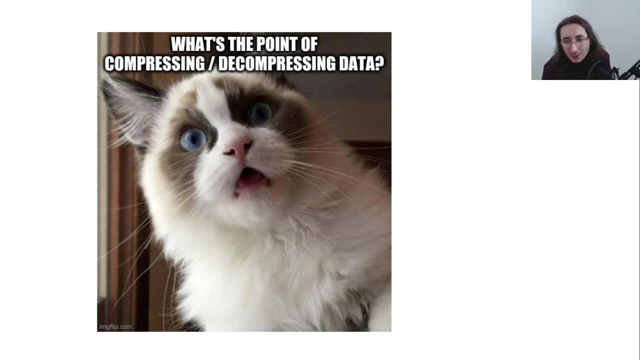 important question, which is: Valerio, but why are you teaching us about like this incredible architecture where you start with data, you compress it down and just then to decompressing back, like to the original data? So what's the point of that? Can we just use the input data? I mean, why do we? 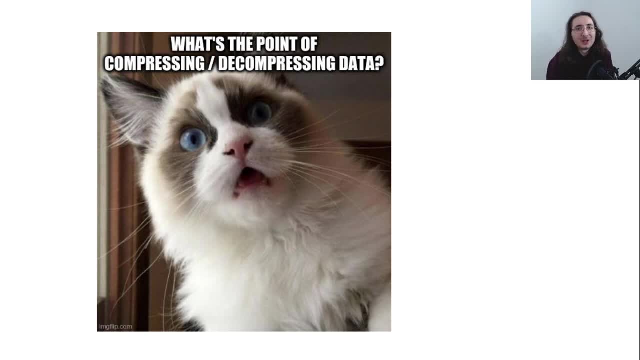 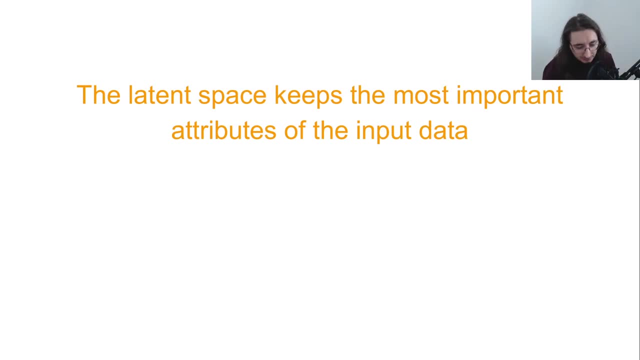 need the reconstructed data? Why do we need compression at all? Well, there's a reason for that, and the reason is the latent space, And the latent space, as we've come to learn, keeps the most important attributes of the input data. Now, having this compressed version of the original data turns 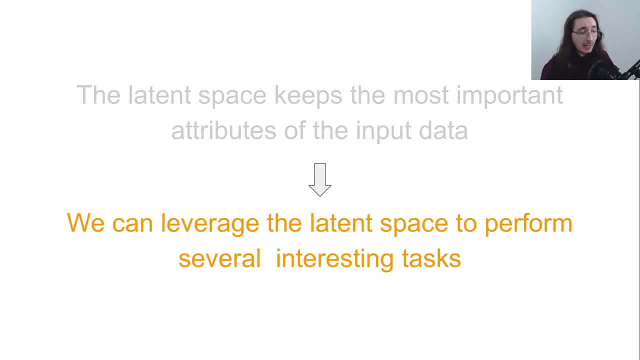 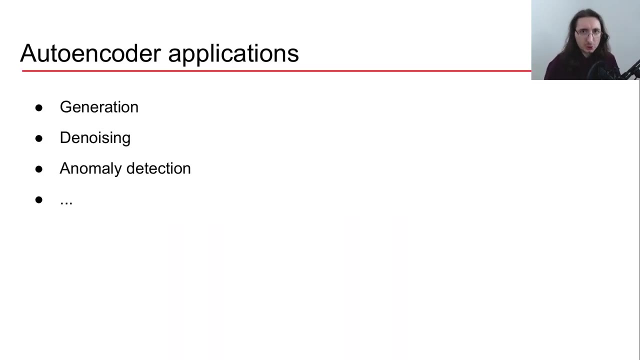 out to be very useful for performing a number of different interesting tasks. Now let's take a look at a few of these. So we can use autoencoders for generating data, and obviously that's what we're going to do, like in this series, and it's the whole point of choosing autoencoders for this. 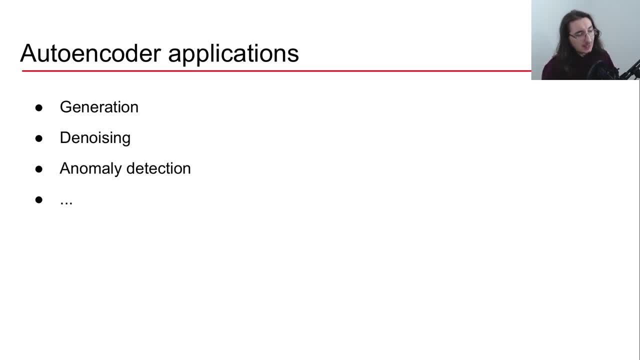 series on sound generation with neural nets. right, Then we can use autoencoders for denoising data and we can denoise images, we can denoise sound- whatever we want really. And then we can also use autoencoders for anomaly detection, detecting anomalies or malfunctions, for example, in a machine. 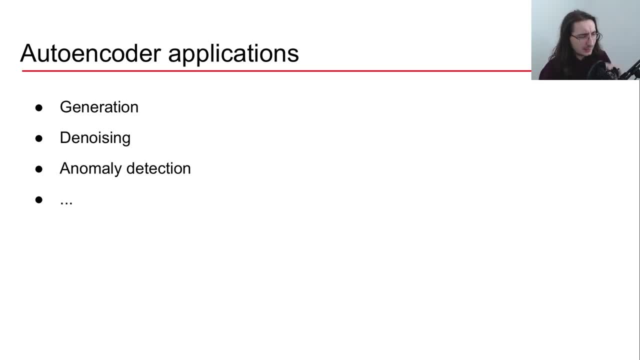 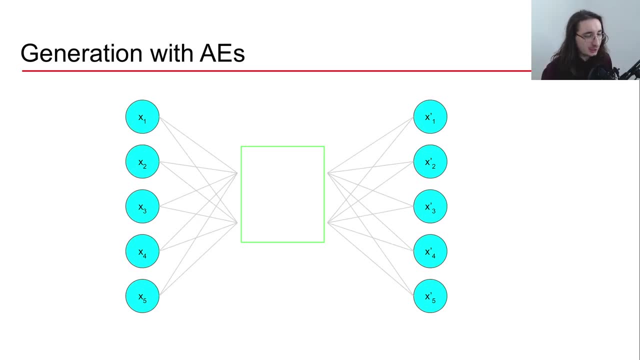 And there are a bunch of other applications that I don't want to get into right now. Let's take a look at generation first, with autoencoders. So here we have once again a visualization of an autoencoder, but the bottleneck is slightly different, because now I want to have, like I, 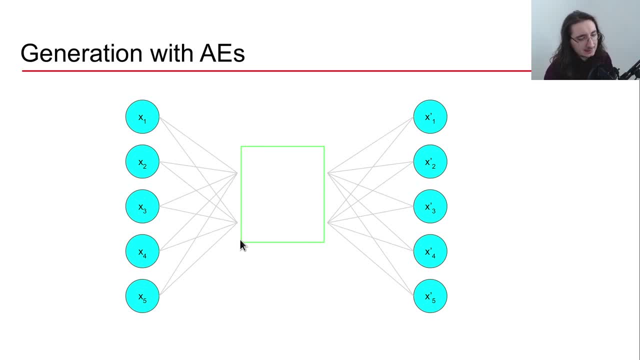 said: I want to have a 2D plane or a 2D space. So you can imagine, this is the x-axis and this is the y-axis. Okay, so now let's see what happens once we train an autoencoder. Basically, the idea is: 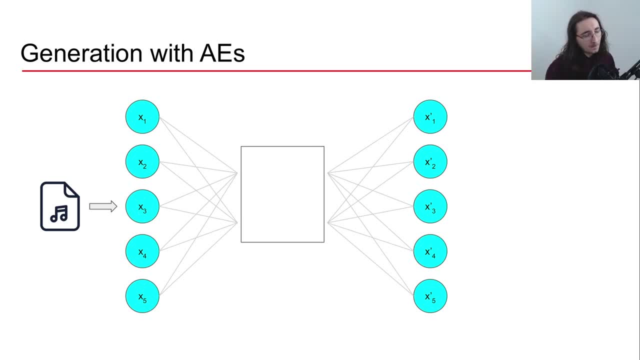 that we can feed some data into the encoder, and obviously here we can feed any type of data. It could be an image, it could be a raw audio, it could be a spectrogram. For the sake of this example, let's assume we are feeding in. 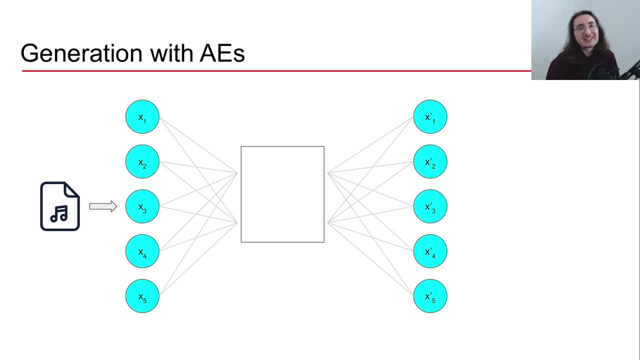 some spectrograms. that's convenient because it's what we'll be using throughout this series for generating sound in the end. Okay, so we feed like these spectrograms into the encoder and then the encoder will encode the original spectrograms into a point within this. 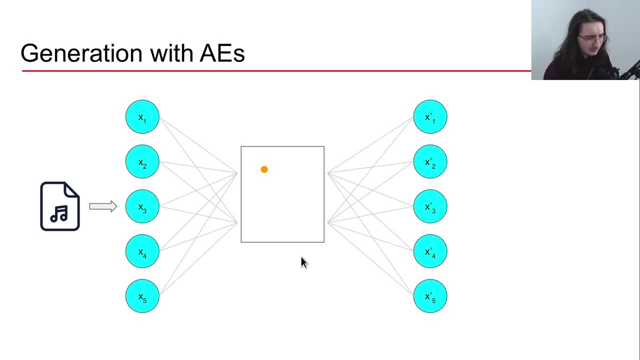 two-dimensional space or the latent space. Okay, now what's gonna happen is that when we feed this point into the decoder, hopefully the autoencoder- or the decoder in this case, is gonna be able to reconstruct the spectrogram and this reconstructed spectrogram, hopefully, is gonna be very similar to the original spectrogram. that 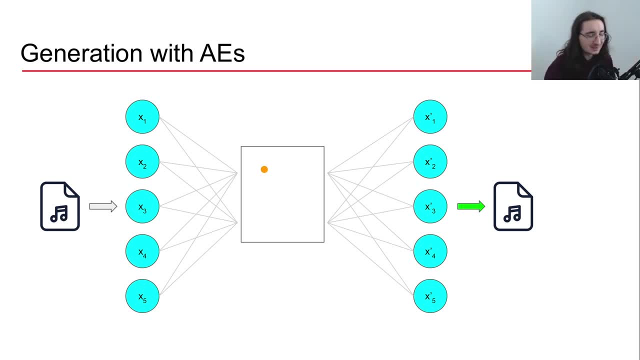 we fed as input into the encoder in the first place. okay, so now if we feed another spectrogram, a new spectrogram, probably we're gonna have like another point, say here, like in the latent space, and let's assume we feed a third one and the fourth one and the fifth one, so, as you can see, like all the input. 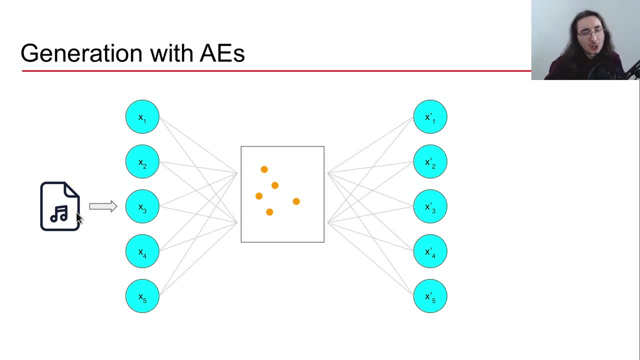 spectrograms that we feed into the encoder gets mapped onto a point in the two-dimensional latent space. okay, so now we've learned a representation of the spectrograms and all the inputs that we fed into the network. okay, so now how do we generate stuff? well, first of all, we can drop the encoder part, because 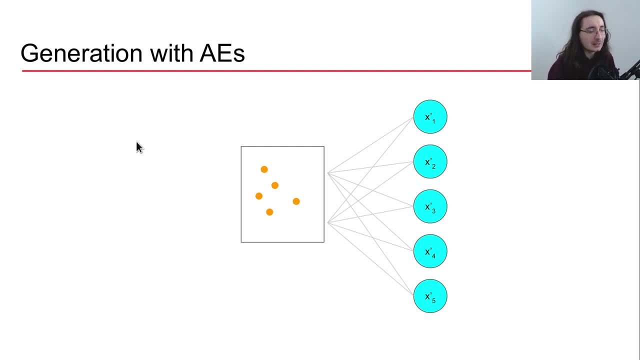 we don't need that for generation. what we actually need is the latent space, so the representation that we've learned, as well as the decoder. so here the basic intuition is that we can sample a new dot in this latent space that's different from all the other dots that we've. 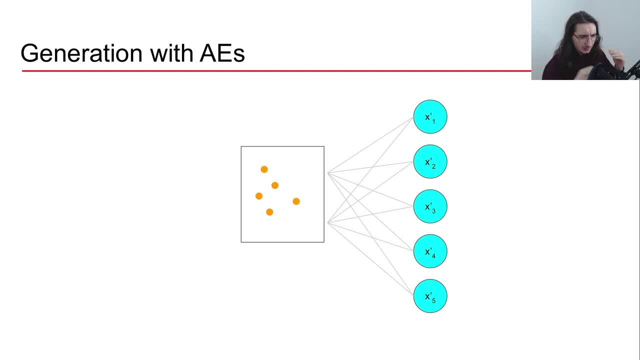 learned or that we've encoded at learning to a training time and that dots can be used to generate a new spectrogram. so how do we do that? well, we sample dot, let's assume like it's this green dot here, and then we feed that into the decoder and hopefully the decoder is gonna generate a new. 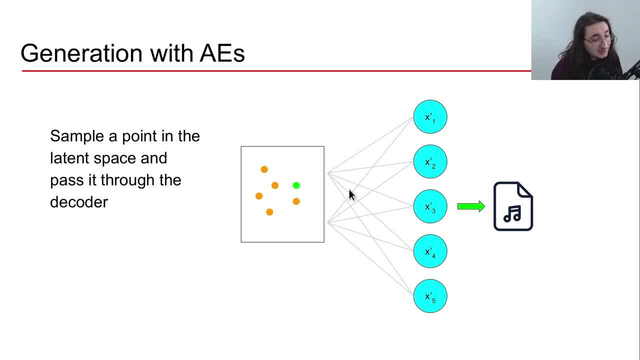 spectrogram. that makes sense. but now, since we've sampled a dot that's different from all the other dots- like that we've learned during training- the spectrogram that we output is gonna be different from all the other spectrograms, and so we are generating new data. so basically, the idea here is: 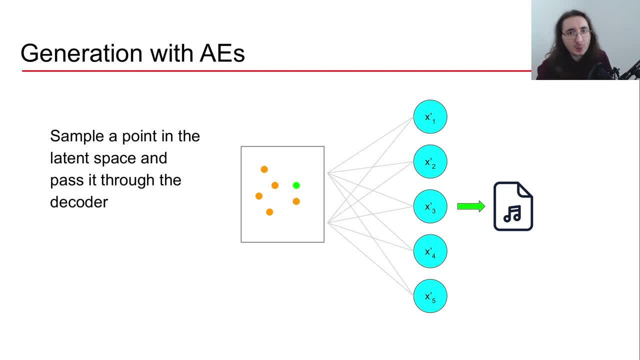 that we can use the latent space and sample it and sample points in there, pass this through the decoder in order to generate a new data, and then we can generate new spectrograms or new images or new raw audio, depending on the different types of like data we've used for training. okay, now, this is not. 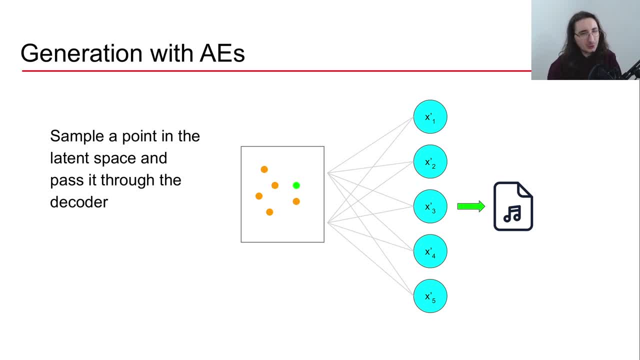 this is not gonna be like this simple with autoencoders, because they have, like, certain limitations, but the basic idea that we are using here for generation with autoencoders is the one that we'll actually use in the upgraded version of an autoencoder, which is a variational autoencoder. so if you want to learn more about, like all, 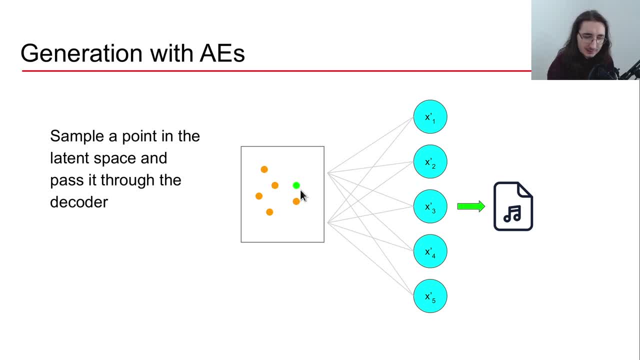 the kind of limitation of autoencoders and why this is not necessarily so easy. so, like this process is not necessarily so easy, let's use with autoencoders. so you have to wait for the next video where we'll see autoencoders limitations. once we create autoencoders, once we code it, let's move on. 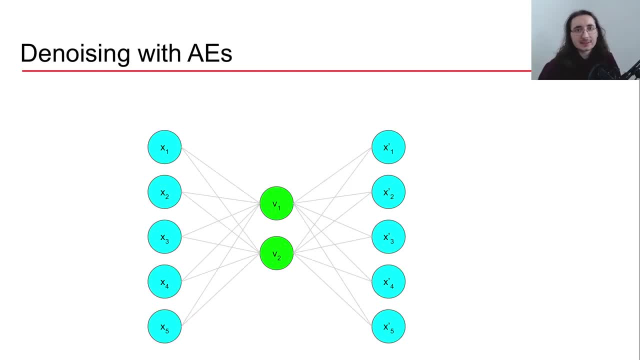 to denoising. so let's see how we can denoise data using autoencoders. here we are back to the original visualization that we used of autoencoders. now we can denoise any type of data- audio images- but obviously we'll be using audio as an example here, so what we want to do is start with some. 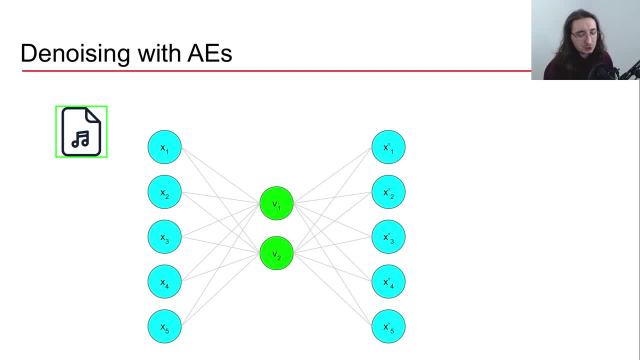 normal, like audio. the next step is to add some kind of noise to that audio file, so it could be like white noise, it could be like the noise of a car engine, you name it really, but the basic idea is that we want a corrupted version of the. 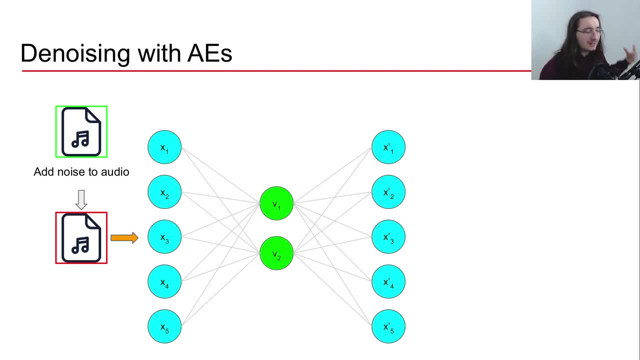 original audio and this is what we're gonna be feeding into the network. but basically the idea is that what we want at the output of this network, of this autoencoder, is a reconstructed audio that's gonna be equal to the original audio, that's basically without any noise. so how can we obtain that? so, because, like that, 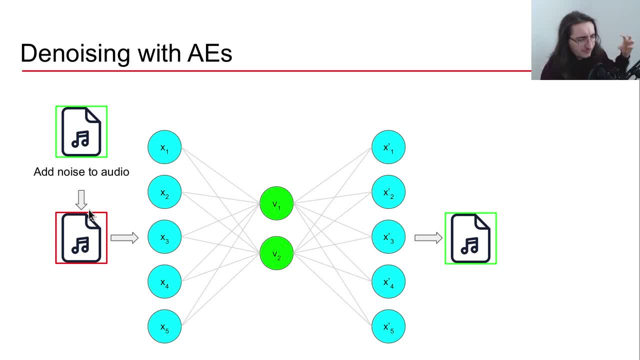 sounds like really difficult. so we start like with. so we feed like noisy data, noisy audio, and then we expect for, for the network like to come up with like the original audio without noise. well, it all depends on the reconstruction error that we'll use. in other words, we'll measure the reconstruction error. 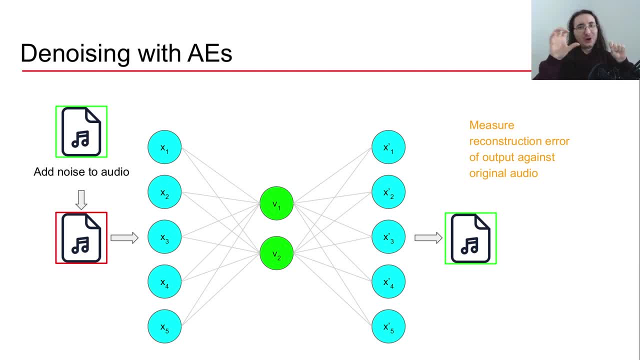 of the output against the original audio, right? so instead of, like you create, having like the reconstruction error being the difference between the output and the noisy input, will have the difference of the output with the original audio, without noise, and so yeah, yeah, yeah, this sounds like really. 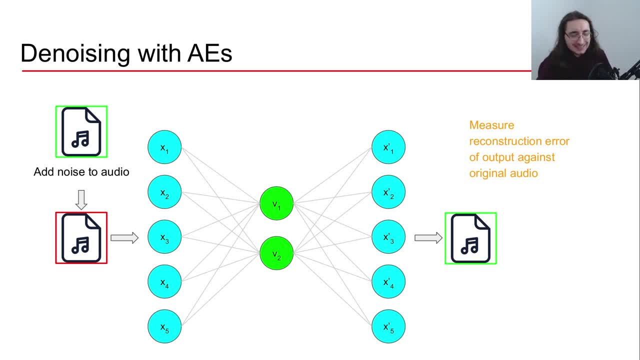 interesting, but how can like an autoencoder then, like denoise? well, the point once again is this bottleneck is the latent space. so what we are hoping to do by using, like this reconstruction error, which like these two elements, so the output and the original audio, is to capture the most important, the features. 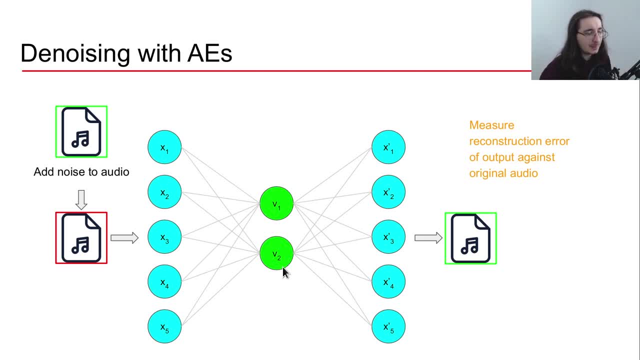 of audio and encode them here in the latent space and leave out the unnecessary details or unnecessary features like noise, for example. so the the hope is that we are going to learn a representation here in the bottleneck that focuses only on the, the part of the signal that we are 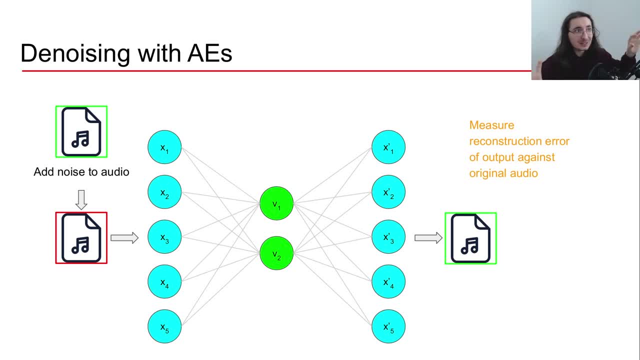 interested in and leaves out the, the noise that we actually want to cancel. so then, basically, the idea is that we start with, like a noisy signal with the, we encode it down in the latent space and that representation, hopefully will leave out, like the, the noise, and then, when we pass it through the decoder, hopefully, 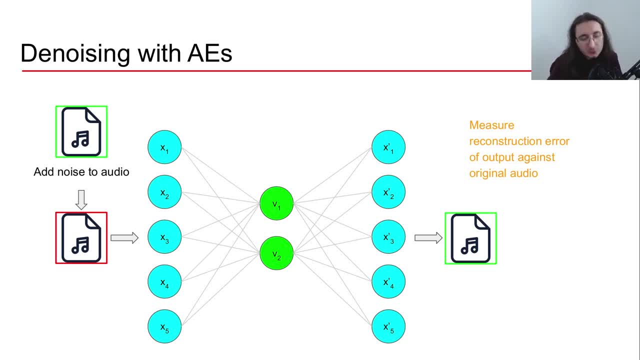 we'll get back like an audio file that's sounds like more like the original than its noisy version, right? so here you see once again how important it is to have a good representation, a good latent space that focuses on the most important features of our and leaves out the unwanted details. 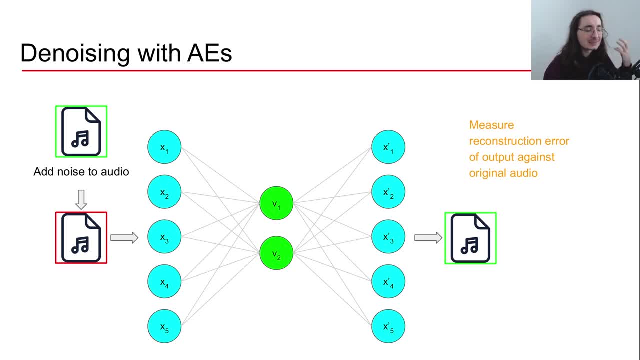 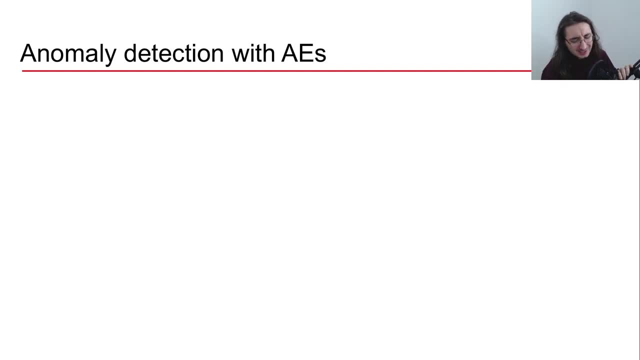 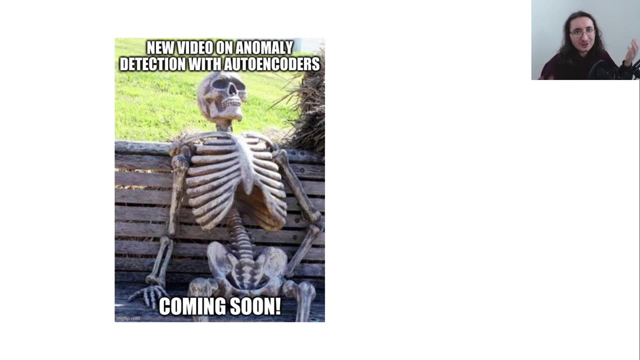 Cool. So this is for denoising. So the last application that I want to talk about is anomaly detection, which auto-enquires, But in reality, I'm not gonna talk about it right now because I'm planning to publish a new video.